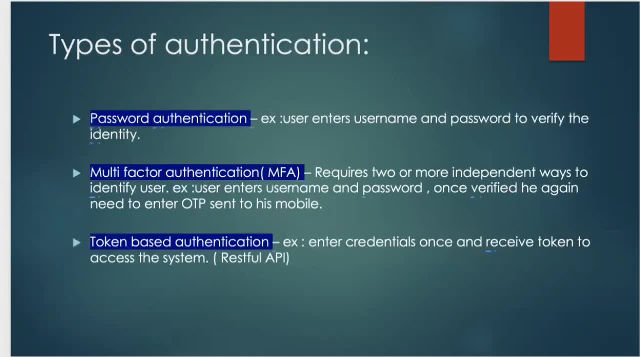 Okay, let's see different types of authentication. We have password based authentication, We have password based authentication, We have multi-factor authentication, We have token based authentication And we have certificate based authentication. We have biometric, We have single sign on, So basically password. 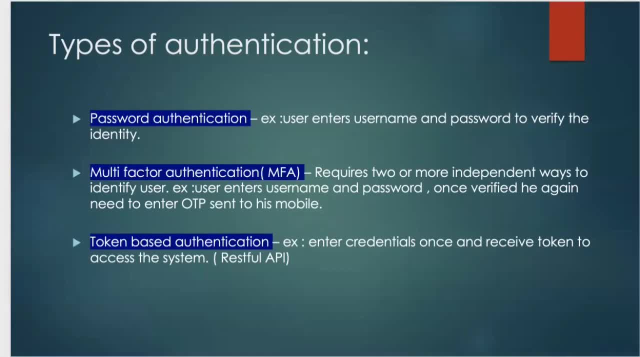 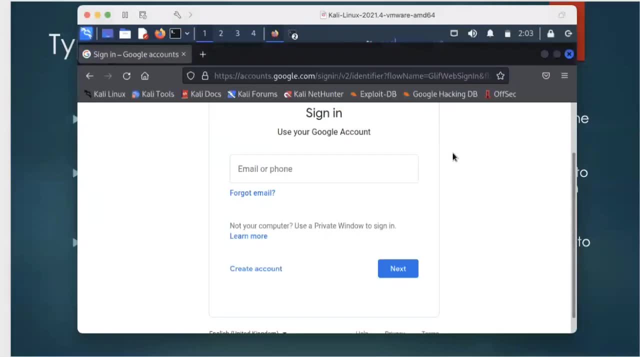 based authentication means, like user enters username and password to verify the identity. For example, you go to Googlecom correct- To log into your Google account. There you enter your username and the password, correct, Okay, Okay, Okay, Okay. 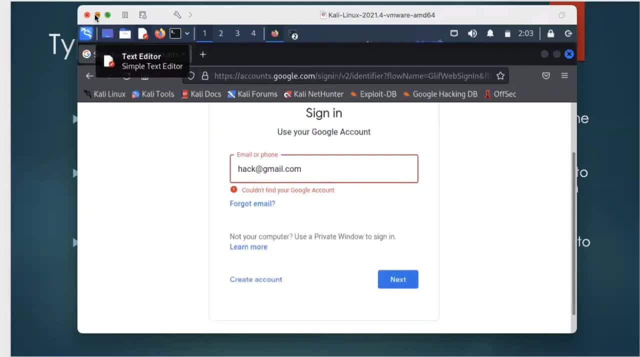 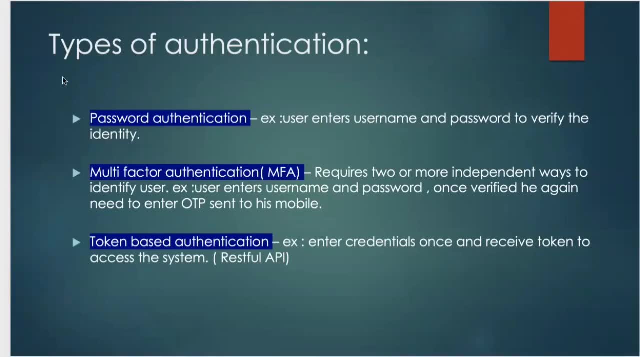 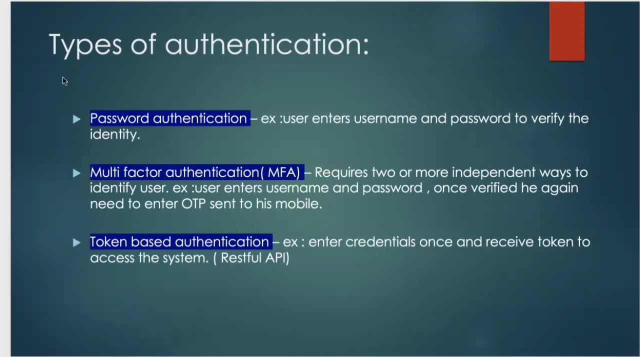 OTP to your mobile, correct? So if you enable two-factor authentication in the Google account, so it will happen. So you need to enter username and password as well. So it basically strengthens the security And we have next, we have a token based authentication example. So basically, user will enter the. 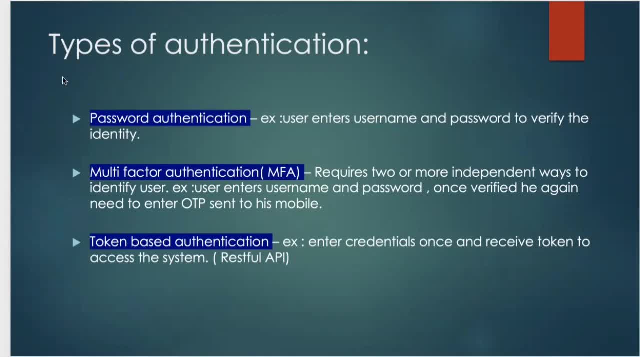 credentials only once. Once he verifies with the credentials entered he will get a token. So using the token he can authenticate to the system afterwards. So only he need to enter the credentials once, So no need to enter it every time. Token based authentication example is Threshold APIs. So when API makes a request, so they 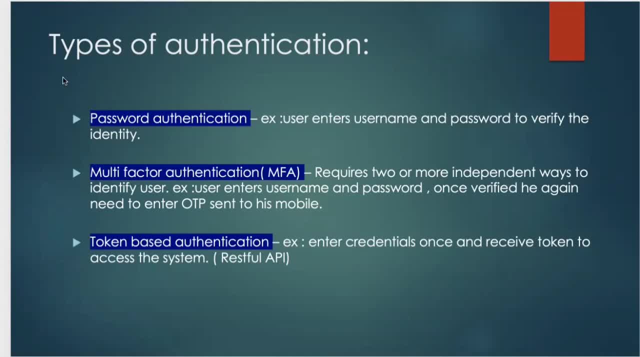 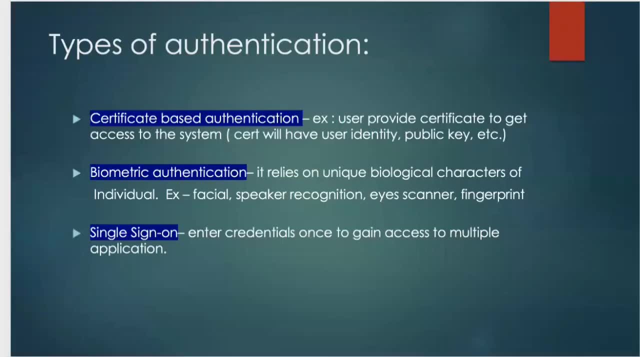 basically authenticate using the tokens: Yeah. certificate based authentication: basically, user will provide a certificate to the system so that it can authenticate. It can identify the user user identity and grant access based on that. So the certificate, digital certificate- will have the user identity information. 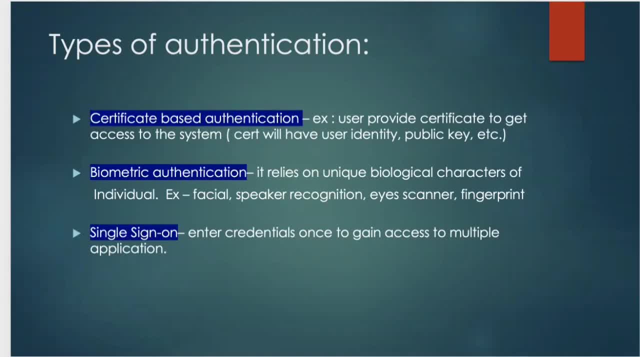 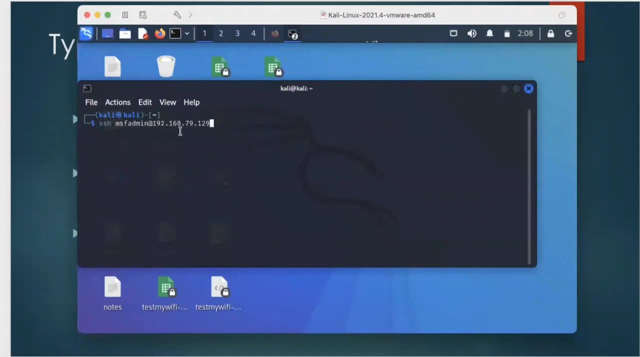 It will have the public key and it will have other information also. So, for example, if you are authenticating to a server like you can do that using certificates. I'll show you the example. For example, I'm connecting to this server 192.168.79.129 using the SSH.